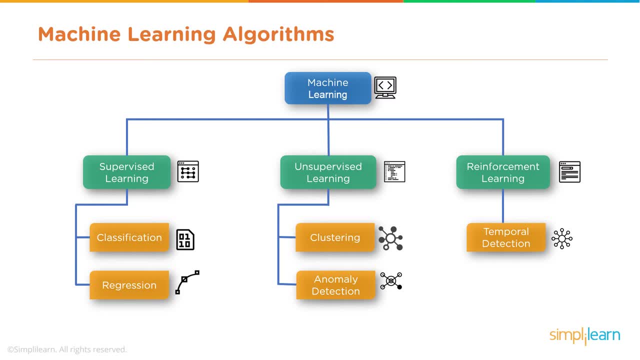 And today we'll cover classification under supervised learning. Supervised meaning the data set has known outcomes. If it were unsupervised, it would not have known outcomes and we wouldn't have the categories or classes necessary for the machine to learn. But under supervised learning we do have the known outcomes in the data set. 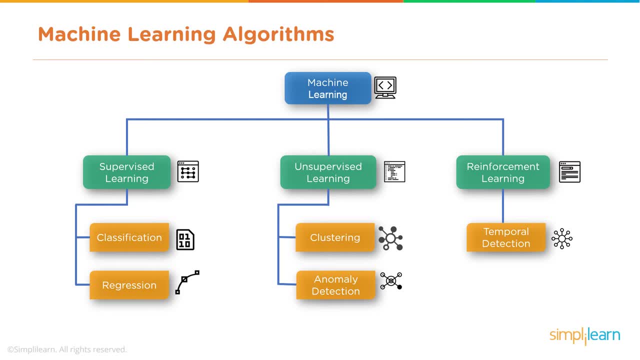 And under supervised learning. there are two major types of machine learning algorithms: Classification, which we'll cover today, Support Vector Machine And regression Classification: you predict categories And in regression you generally predict values. So while we look at supervised learning, keep in mind that classification can really be considered multidimensional. 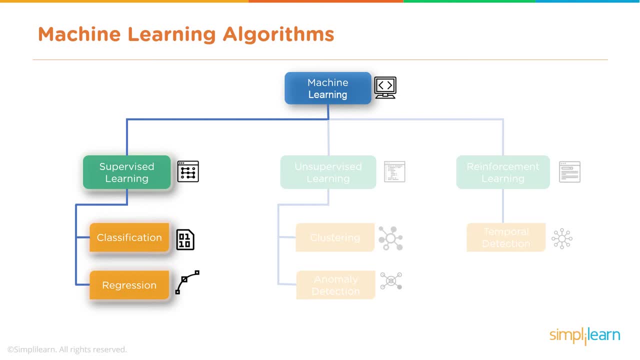 In the sense that sometimes you only have two classes- yes or no, true or false- And sometimes you have more than two classes. Sometimes you have, say, under risk management or risk modeling, Low risk, medium risk or high risk. 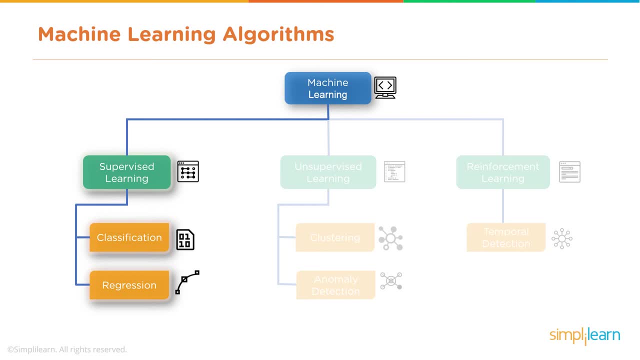 And SVM is a binary classifier. It is a classifier used for those true-false, yes-no types of classification problems And in supervised learning, features are important. If there are a lot of features, SVM may be the better classification algorithm choice, as opposed to say, logistic regression. 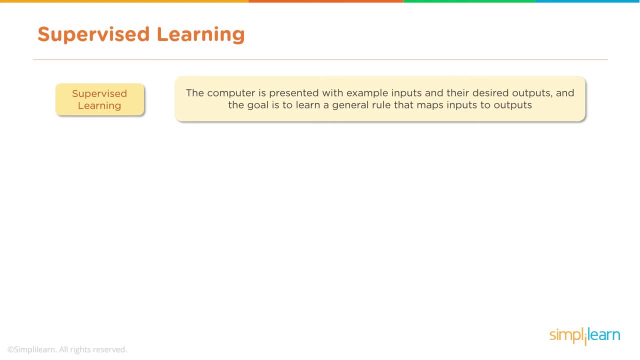 So, for supervised learning, the computer is presented with examples, Inputs and their desired outputs, Those known outcomes, And the goal is to learn a general rule that maps inputs to those outputs, For example bug detection or customer churn, or stock price prediction. 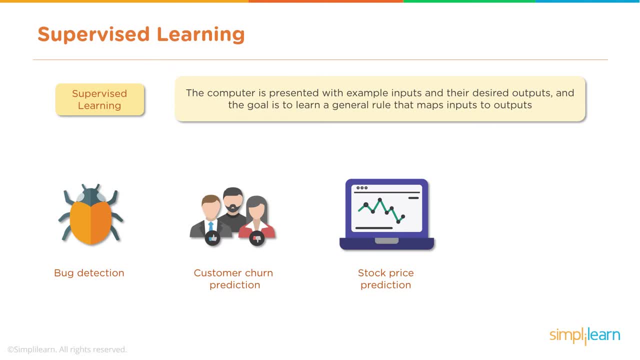 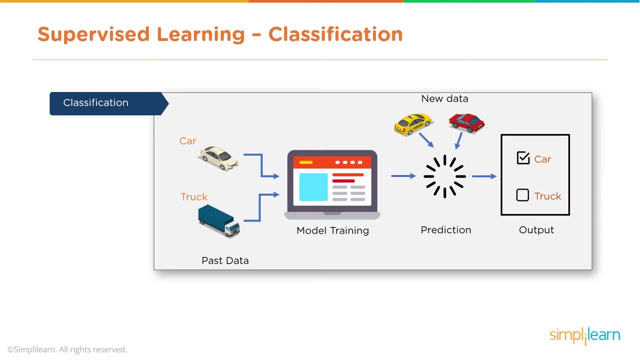 Not the value of the stock price, but whether or not it will rise or fall. And weather prediction: Sunny, not sunny. Rain, no rain. Well, classification algorithms generally take past data, Data that we have, those known outcomes. Train the model. 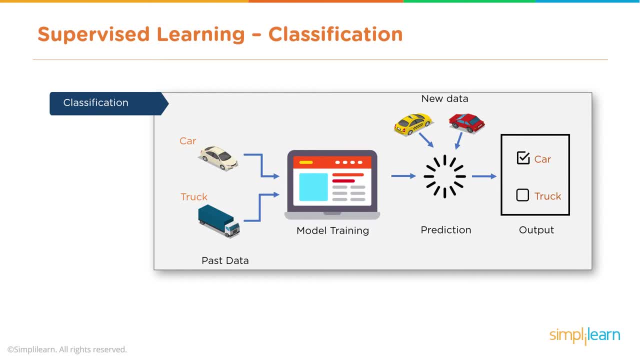 Take new data once the model is trained, Ingest it into the model And create predictions. Is it a truck or is it a car? And keep in mind that I said, features are important And the number of features, whether or not those features are applicable to your problem, is a whole different discussion. 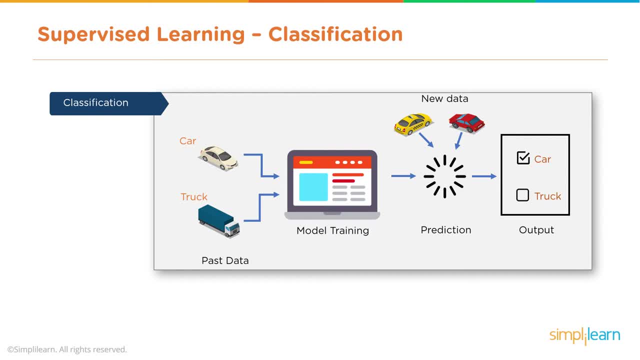 But in some sense you know, probably intuitively, that the color of a car really isn't indicative of whether or not it's a car or a truck, But the length of the vehicle or the number of axles Or the weight or the amount of seating may be more applicable to the algorithm and to training the model. 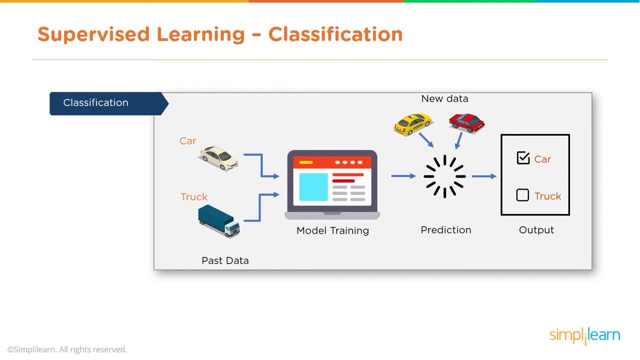 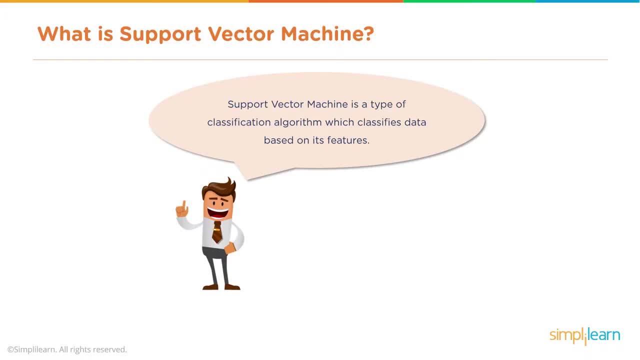 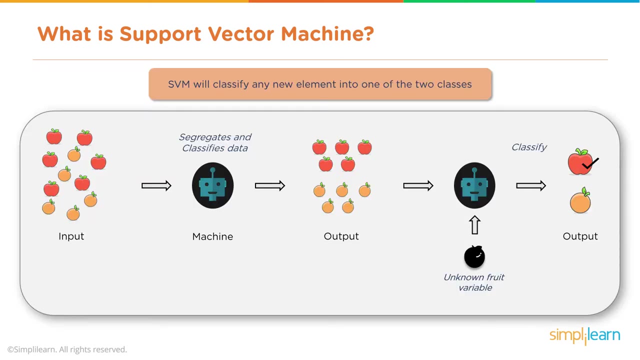 So what is support vector machine? Support Vector Machine, or SVM, is a type of classification algorithm which classifies data based on its features, And SVM will classify any new element into one of those two classes. So we'll give it some inputs. 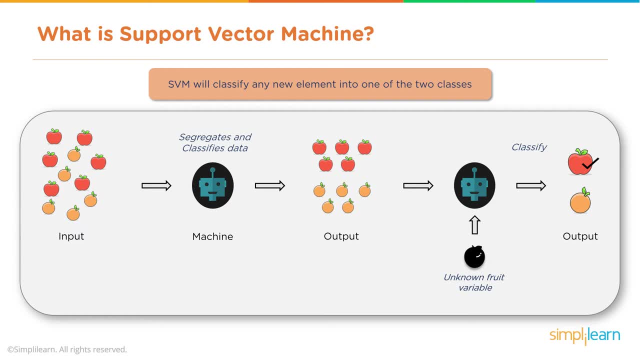 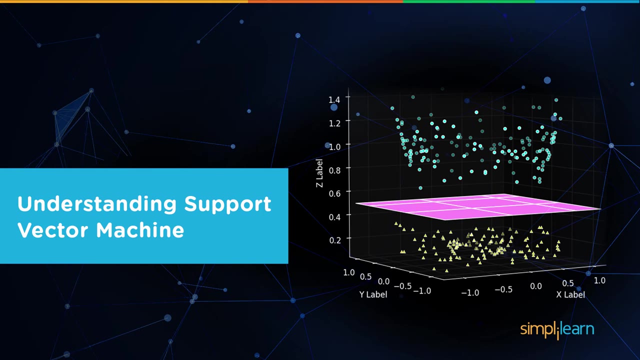 The algorithm will segregate and classify the data and then create the outputs And next, when we we ingest new data- an unknown fruit variable in this example- the algorithm will correctly classify the fruit apple versus orange. So now let's understand what an SVM is and if you want to, 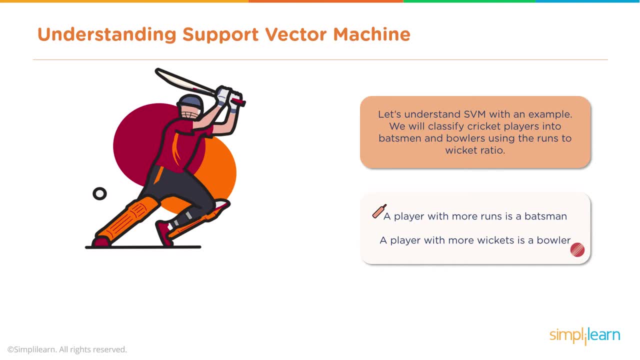 understand support vector machine. you really need a good example, and I know that cricket is a wonderful game. I don't know a lot about it, but I know it's very popular around the world and we're going to use cricket as an example of SVM, So we'll classify cricket players into batsmen or bowlers. 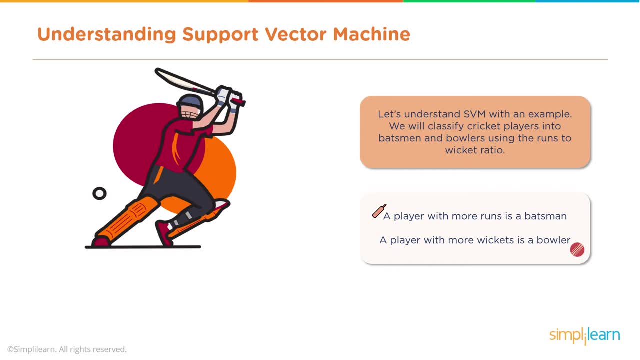 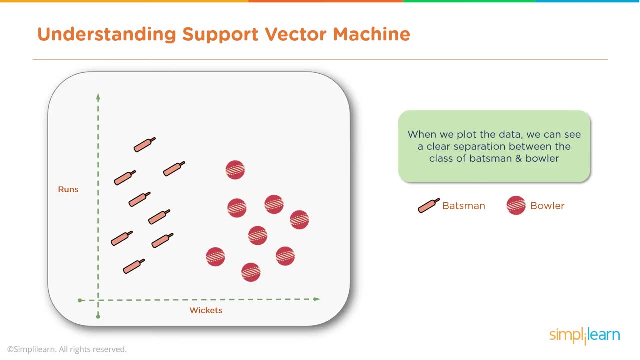 using the runs to wicket ratio. So a player with more runs would be considered a batsman and a player with more wickets would be considered a bowler. and if we could take a data set, say, of people- cricket players- with runs and wickets in columns next to their names, we could create a 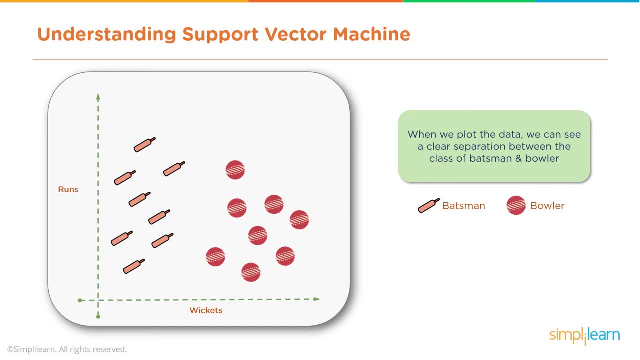 plot, a two-dimensional plot in this example, Clear separation between cricket players considered bowlers and those cricket players considered batsmen, and you don't always have a data set this clean where there is a clear segregation of data: bowlers versus batsmen. but for the sake of understanding SVM, this example does well. So 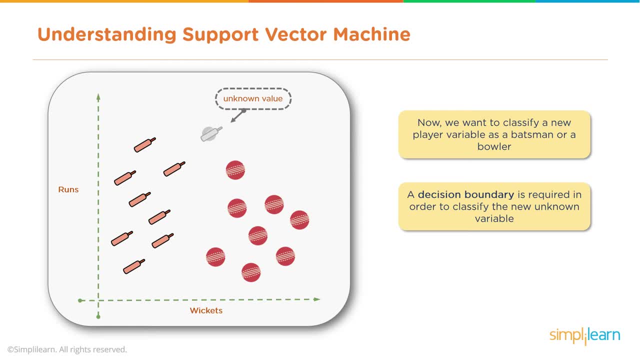 before we do any separation, before we apply any high-level mathematics, let's just take a look at an unknown value, a new data coming into our data set, And that datum- we don't know what class it belongs to. That datum is a bowler or a batsman, we know. 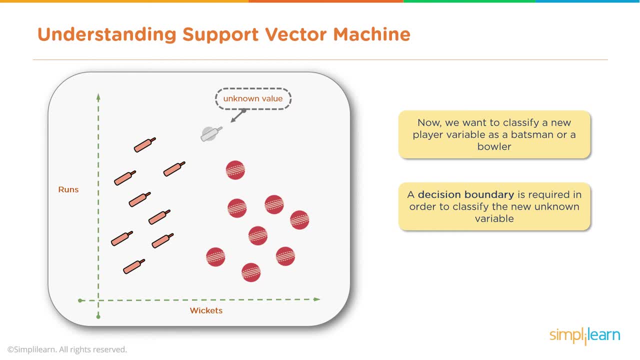 that much. but we don't know should we consider that cricket player a batsman or a bowler? and so we want to draw a decision boundary, some type of line separating the two classes, so that we can use that decision boundary to classify the new data point. Of course we could draw lines. there's a. 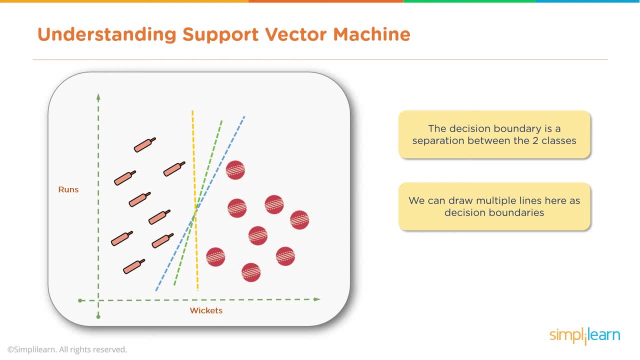 yellow line, a green line, a blue line. there's actually not just a blue line, there's actually a three lines, but an infinite number of lines that we could draw between those two classes. so which one do we pick? and this is kind of reminiscent of simple linear regression, where we find the line of 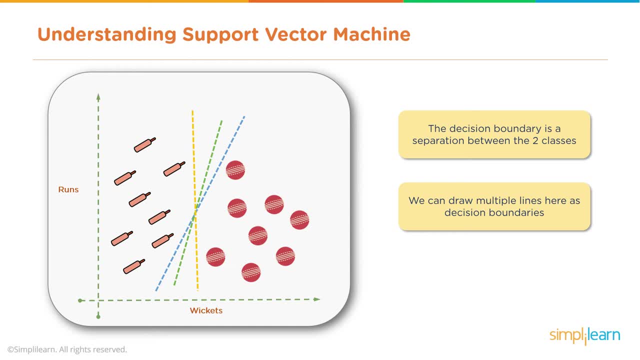 best fit. we want the line of best separation. we want a line that clearly separates those two groups as much as possible. Once we have the correct line, we would be able to classify the new data point. but in this example you can see, if we pick yellow, the new data point would be a bowler. 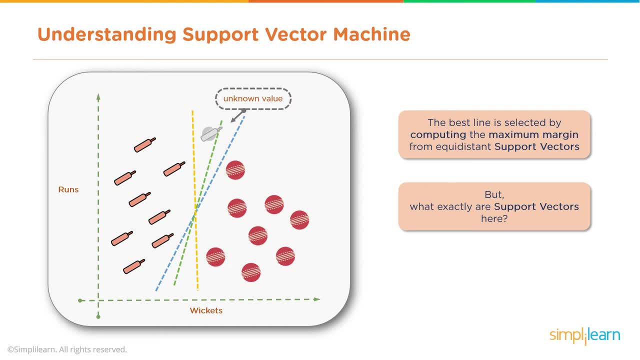 but if we picked green or blue, the new data point would be a batsman. so we need the one that best separates the data. What line best separates the data? We'll find the best line by computing the maximum margin from equidistant support vectors. Now, support vectors in this context simply means: 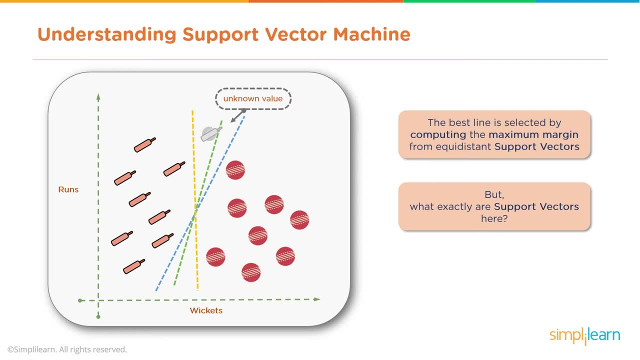 the two points, one from each class, that are closest together but that maximize the distance between them or the margin. So the word vector is a word that means the distance between two classes. So the word vector here you may think, well, he really means points, data, points. well, in two. 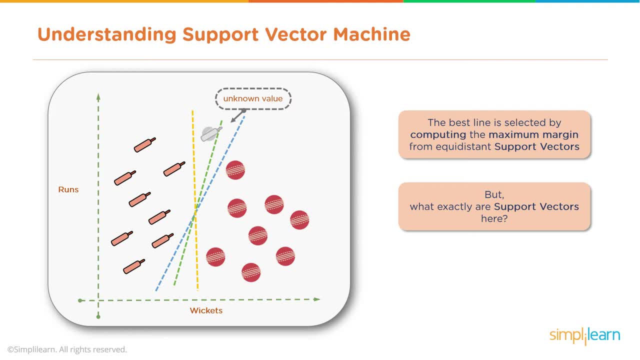 dimensional space, yes, and maybe even in three dimensional space. but once you get into higher dimensional spaces, when you get more and more features in your data set, you have to consider these as vectors. you can no longer really describe them as points, so we call them vectors and the 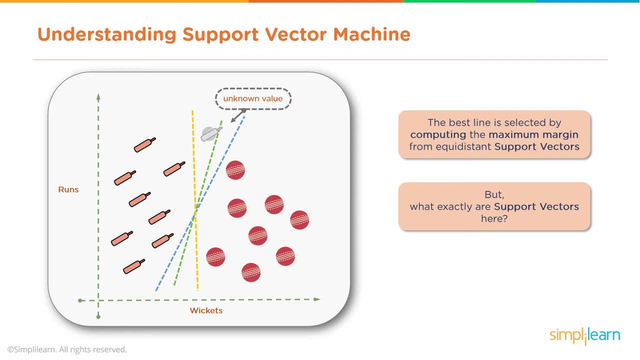 reason they're support vectors is because the two vectors that are closest together, that maximize the distance between the two groups, support the algorithm. so that's why we call them support vectors. So if you look at our example, there are a couple of points at the top that are pretty close. 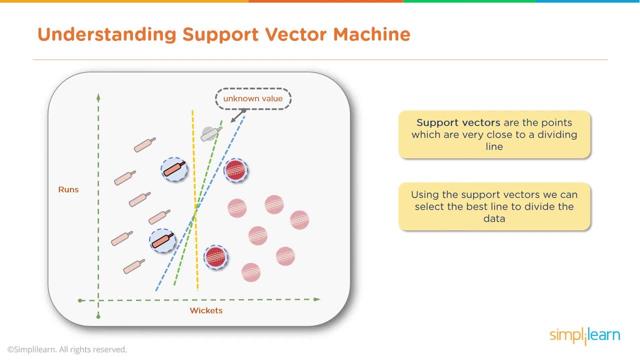 to one another and a couple of points at the bottom of that graph that are pretty close to each other and we're not really sure, looking at the graph, which two are closest, but clearly those points are the ones we need to consider. the rest of the other points are too far away. 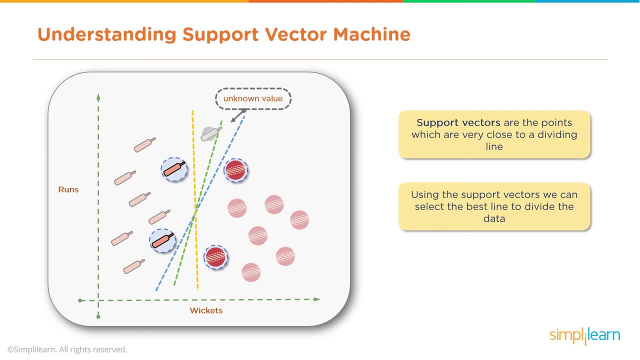 from the rest of the other points. in other words, the bowler points are far to the right and the batsman data points are far to the left. so we'll look at these four points. to begin with, mathematically we would calculate the distance among all of these points and we would minimize. 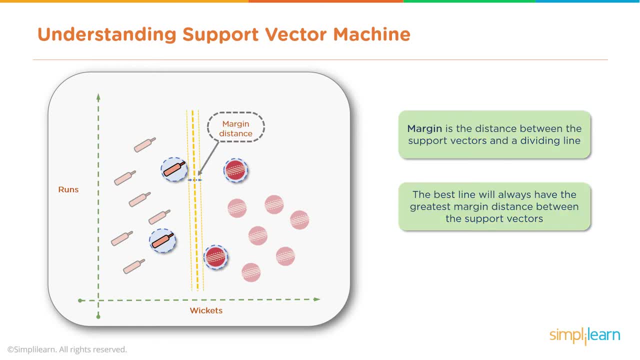 that distance. once we pick the support vectors, we'll draw a dividing line and then measure the distance from each support vector to the line. the best line will always have the greatest margin distance between the support vectors. if we consider the yellow line as a decision boundary, the player with the new data point would be considered a bowler. the margins don't appear. 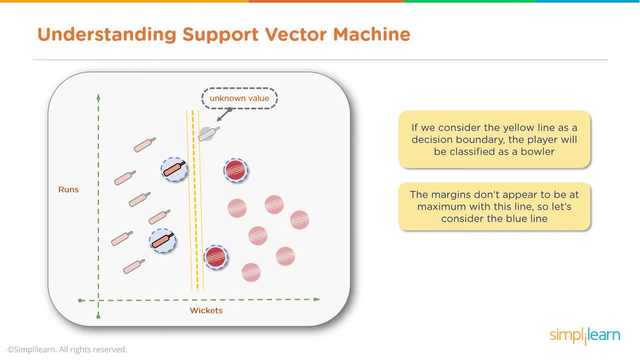 to be maximum though, so maybe we can come up with a better line. so let's take two other support vectors and we'll draw the decision boundary between those, and then we will calculate the margin and notice now that the unknown data point, the new value, would be considered a batsman. we 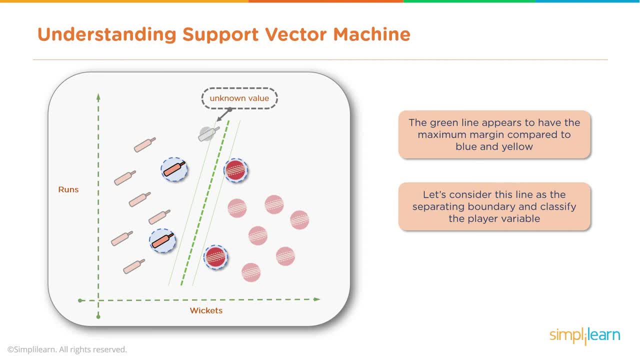 would continue doing this- and obviously a computer does it much quicker than a human being- over and, over and over again, until we found the correct decision boundary with the greatest margin, and in this case, if you look at the green decision boundary, the green line appears to have the maximum margin compared to. 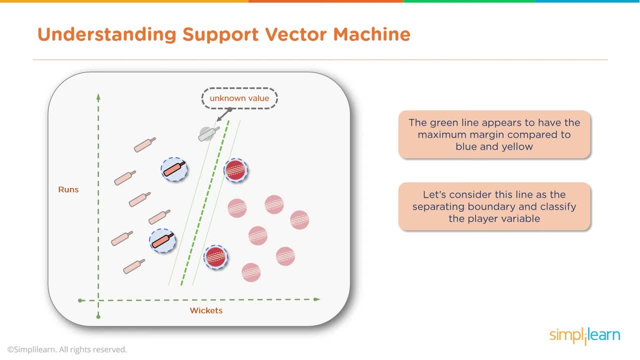 the other two. and so let's consider this the boundary of greatest margin. and now classifier unknown data value. and now, clearly, it belongs in the batsman's class. the green line divides the data perfectly. and then we have the green line, which is the maximum margin compared to the 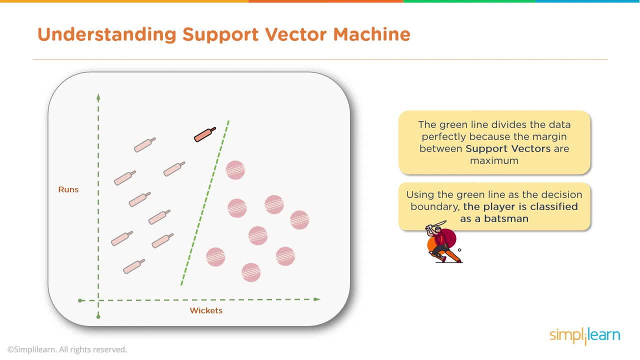 batsman's class. the green line divides the data perfectly because it has the greatest margin, or the maximum margin between the support vectors, and now we can have confidence in our classification that the new data point is indeed a batsman. technically this dividing line is called a. 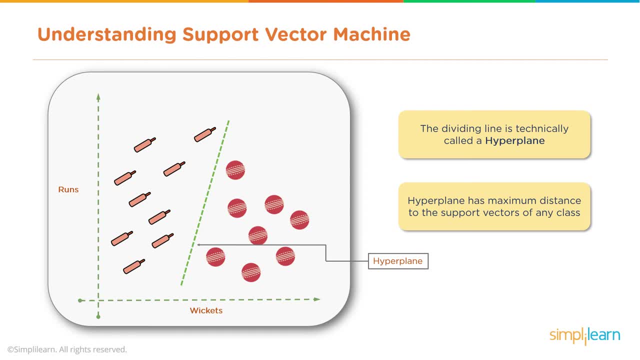 hyperplane and the reason it's called a hyperplane will become a little bit more evident in a few minutes. generally in two-dimensional space we consider those lines, but in three-dimensional space and higher dimensional spaces they're considered planes or hyperplanes, and we can call them hyperplanes. so we always tend to refer to them as hyperplanes, and the hyperplane that has 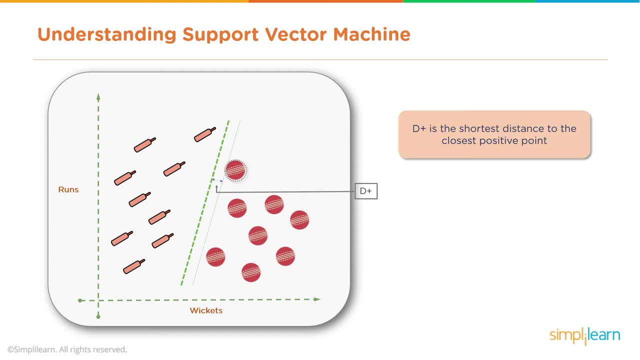 the maximum distance from the support vectors is the one we want. so sometimes called the positive hyperplane, d plus is the shortest distance to the closest positive point and d minus, sometimes called the negative hyperplane, as the closest shortest distance to the closest negative point, and the sum of d positive and d negative is called the distance margin. so if you calculate those two, 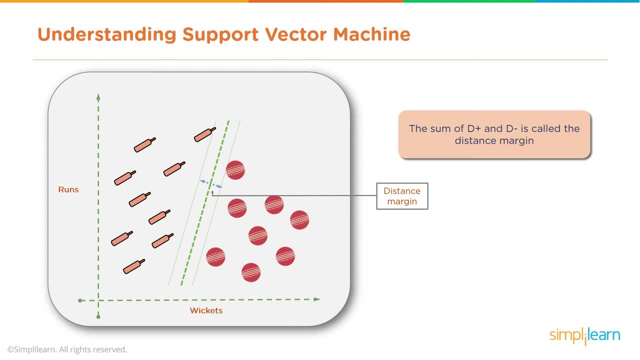 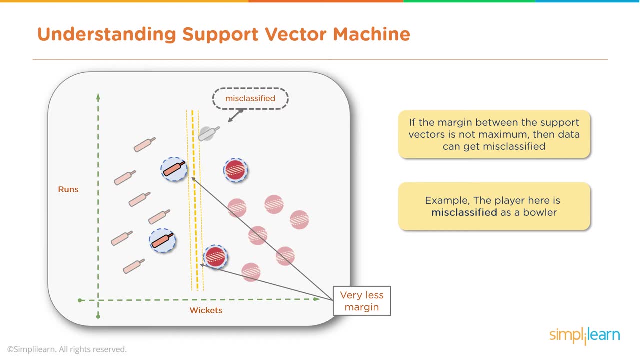 up. that's the distance margin and we always want to maximize that. if we don't maximize it we can have a misclassification and you can see the yellow margin is much smaller than the green margin. so this problem set is two-dimensional because the classification is only between two. 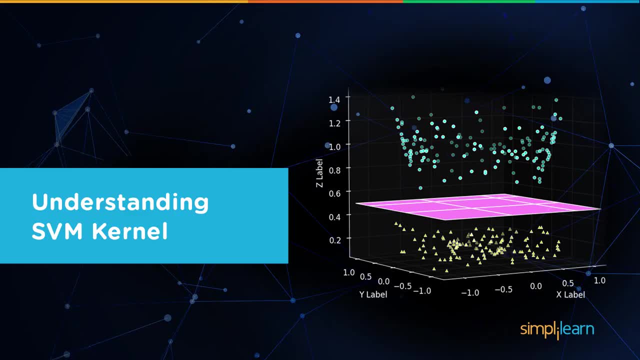 classes, and so we would call this a linear svm. now we're going to take a look at kernel svm, and if you notice in this picture, this is a great depiction of a plane, not a line. this is three-dimensional space, so that's the plane and that's the distance margin, and we always want to. 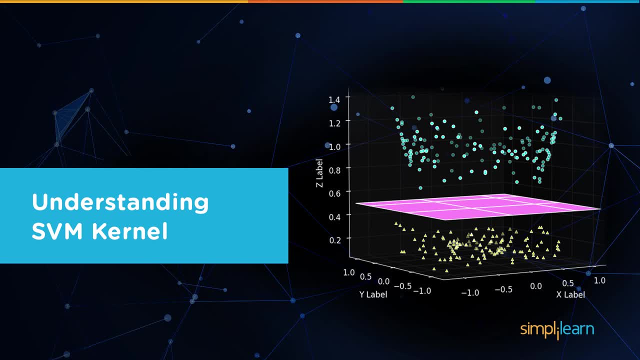 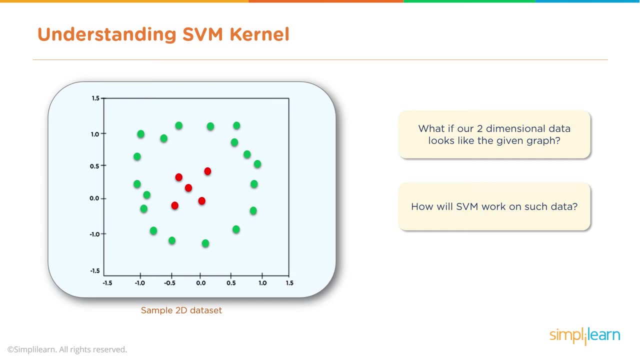 have a line that separates those two classes. so what if our two-dimensional data looks like this? what if there's no clear linear separation between the two classes and machine learning parlance? we would say that these are not linearly separable. how could we get support vector machine? 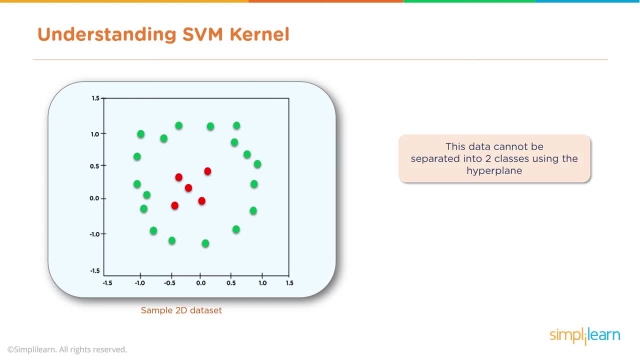 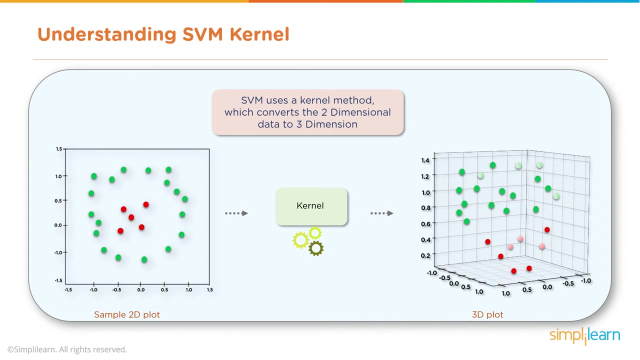 to work on data that looks like this: since we can't separate it into two classes using a line, what we're going to do- and clearly there's no line- i mean, convince yourself, there's no line that goes and separates those two classes. so what we would do is we would apply some type of transformation to a higher dimension. we 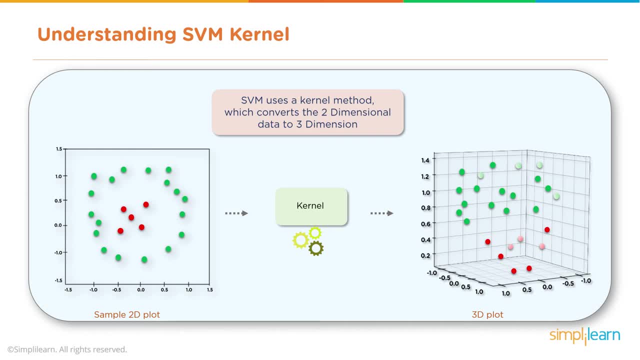 would apply a function called a kernel function to the data set, such that the data set would be transformed into a higher dimension, a dimension high enough where we could clearly separate the two groups, the two classes, in this case with a plane, much the same way. you saw the picture. 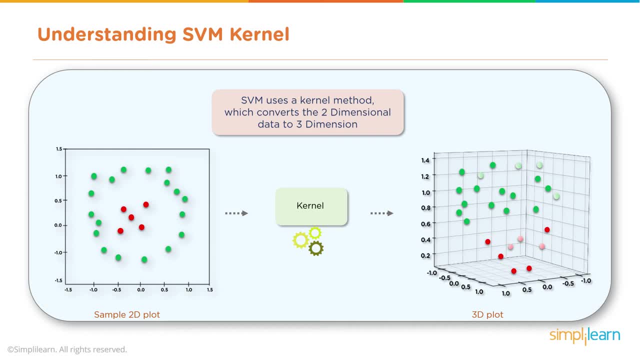 a few slides ago where the plane was separating the two classes. here we clearly could draw some planes between the green dots and the red dots and of course we could draw an infinite number of planes separating those two classes, but we would draw the one that would maximize the margin. 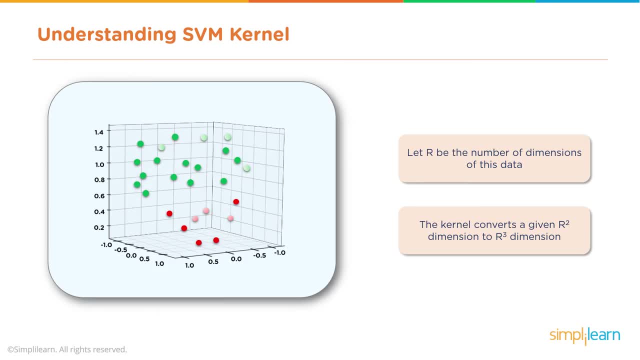 so if we let r be the number of dimensions, then the kernel function would convert a given two-dimensional space to a three-dimensional space and, as i said, once the data is separated in three dimensions, we can apply the kernel function to a higher dimension and we can 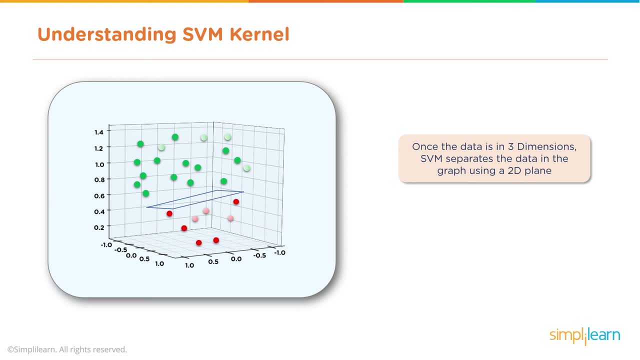 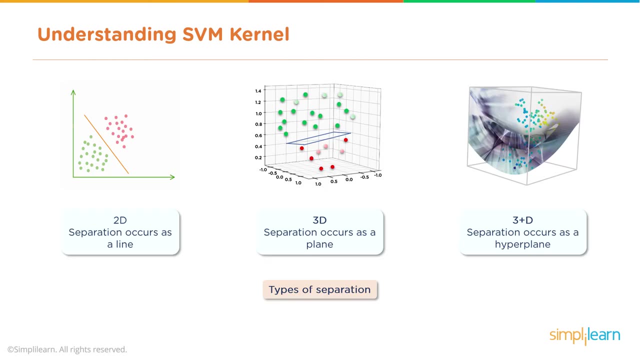 apply svm and separate the two groups using a two-dimensional plane, and this is analogous in the higher dimensions- and that last picture on the right hand side would be some type of depiction of a higher dimension hyperplane- and there are more than one type of kernel function. 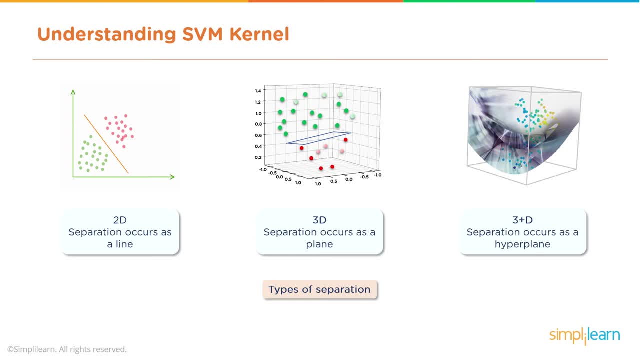 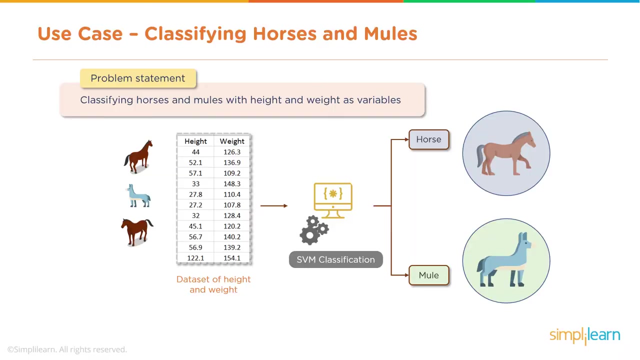 there's gaussian rbf kernel, sigmoid kernel, polynomial kernel, depending on the dimension and how you want to transform the data. there are more than one choice for kernel functions. so now let's go through a use case. let's take a look at horses and mules and see if we can use svm to classify some new data. so the problem statement is: 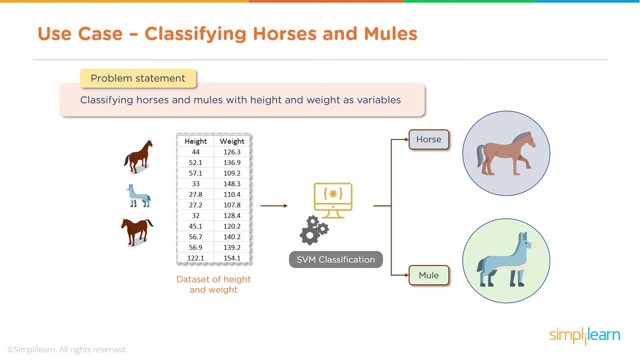 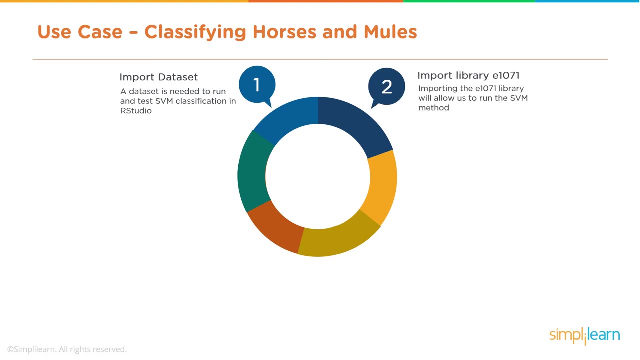 classifying horses and mules and we're going to use height and weight as the two features and obviously horses and mules typically in general tend to weigh differently and tend to stand taller. so we'll take a data set, we'll import the data set, we'll make sure we have our libraries. the e1071 library has. 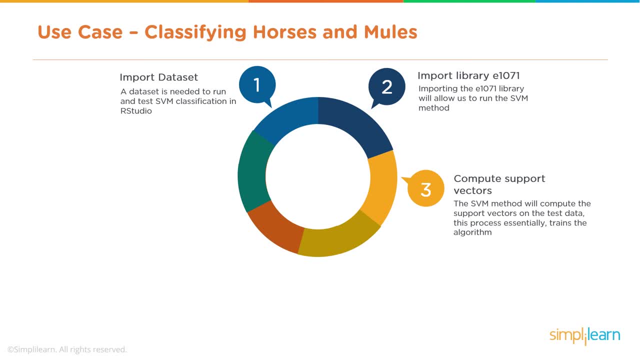 support vector machine algorithms built in. we'll compute the support vectors using the library. once the data is used to train the algorithm, we'll plot the hyperplane, get a visual sense of how the data is separated and if it's two-dimensional or three-dimensional, that's great, remember? if it's. 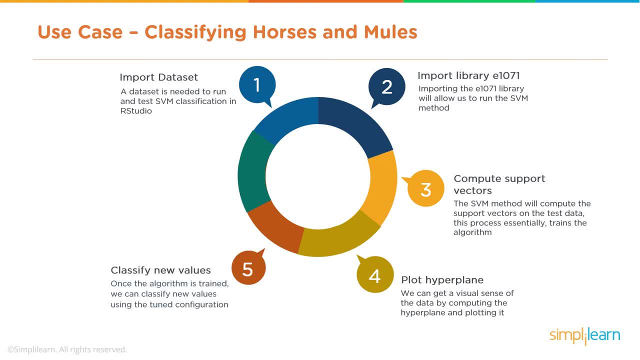 higher dimensional. it's tough to plot those- and then we'll use the new model, the trained model, to classify new values. in general, we would have a training set, a test set and then ingest the data- new data. but for our example we're just going to use the whole data set to train the algorithm and 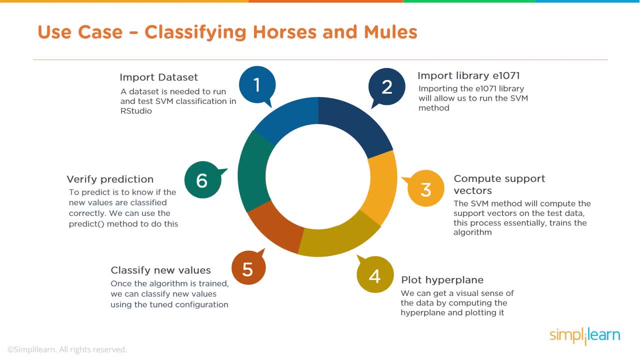 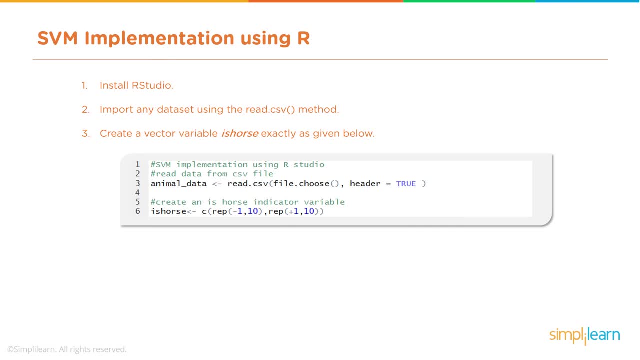 then see how it performs. and once we see how it performs we'll see: did we get a horse? did we predict a horse when we had a horse? did we predict a mule when we had a mule? so here's the r code. of course, if you want to run this r code, you'll have to install r and then r studio. then you'll have to. 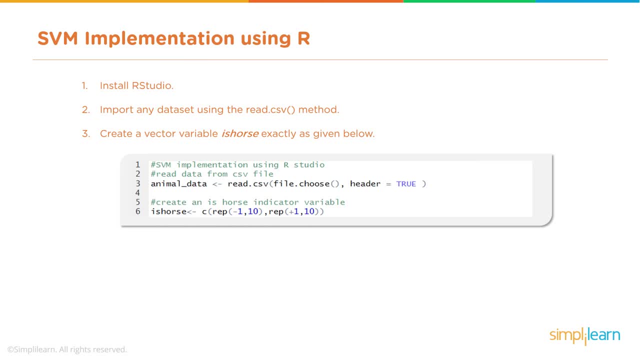 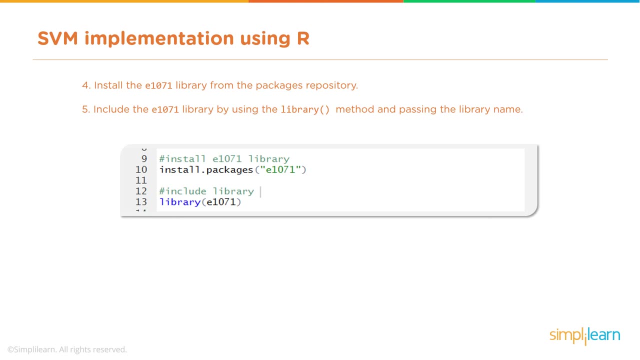 ingest the data and then you'll have to create an indicator variable to help us with our plots. we'll install our libraries. install the package if you don't already have it installed- i do- and then call the library up into the r session that you're working. 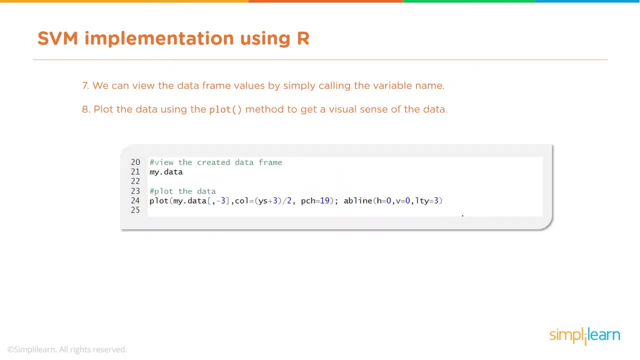 we'll create the data frame from the data that was ingested. we will then view the data frame and, of course, we have to explore the data frame, hoping that we don't have missing values or we don't have outliers. if we do have missing values or outliers, we'll have to either impute those values. 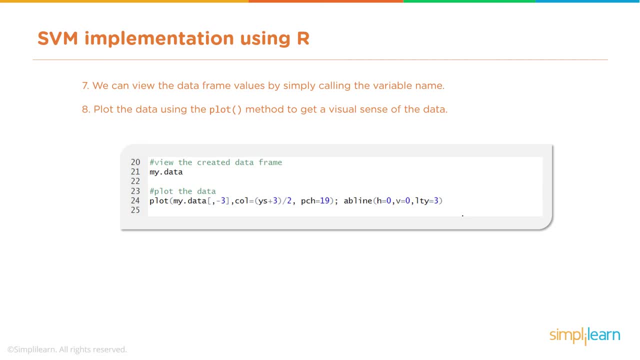 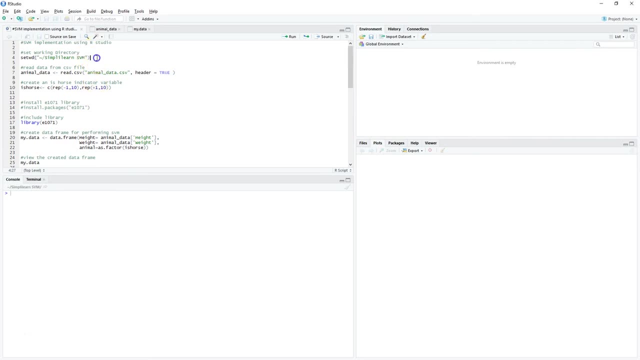 or delete those values, but in this case let's hope we don't have any. and now for a quick demo on support vector machines. so we have a working directory where my data is stored and i'm going to set the working directory to that data source and read the data file into r. and now i'm going to create a vector that really 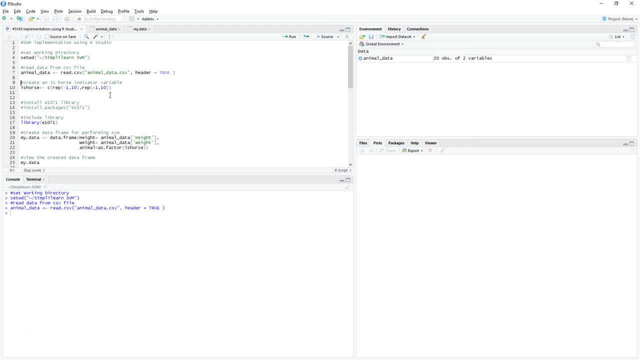 is just an indicator variable. it's the negative ones and the ones that indicate whether it's a mule or a horse- negative one for mule, positive one for a horse. so i'll create that vector and svm. there's a great package: e1071, great library. 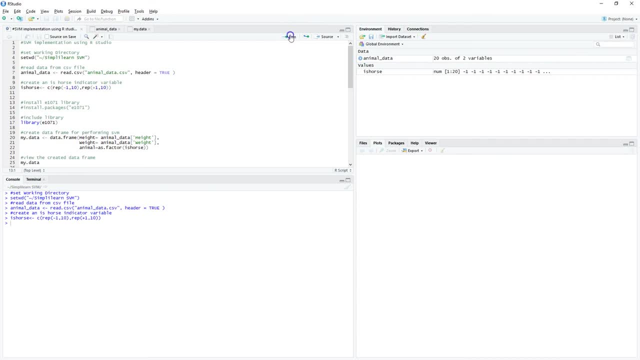 that has the support vector machine functions that we're going to use. and now i'm going to create the data frame. i'm going to take my data and i'm going to add to it the is horse vector. and now let's just take a peek and, as you can see, there's the height, weight and whether or not. 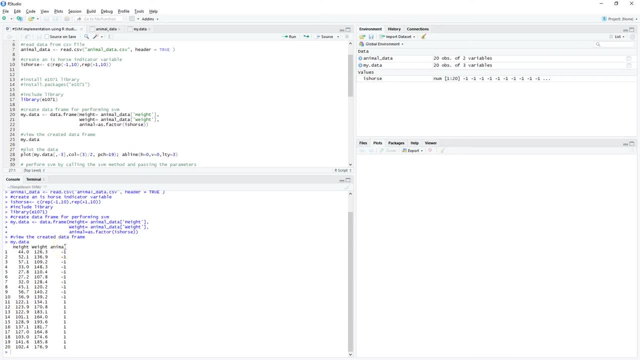 the animal was a mule or a horse. so remember machine learning: we take a data source with known outcomes and we apply our algorithm to that data source, in this case a data frame of heights, weights and the indicator variable, and then we the machine learning algorithm to learn from that data with those known results. 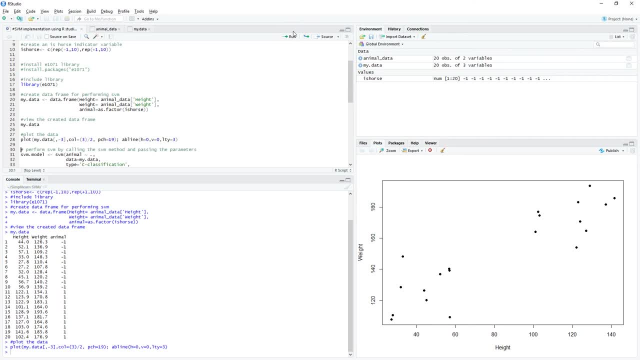 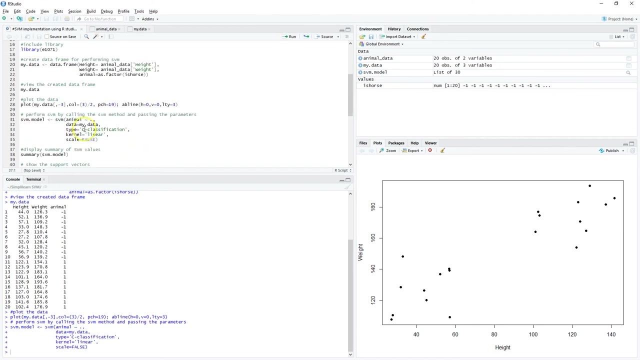 so now let's plot the data, the height versus weight, and, as you can see, the horses tend to be a lot taller and weigh a lot more than the mules. so now let's run our algorithm, our SVM model, against the data, and the key here is that it's a 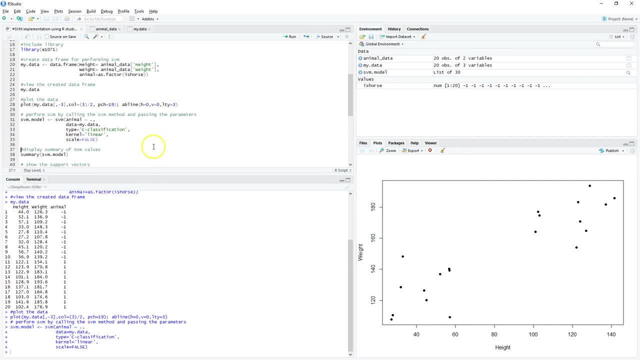 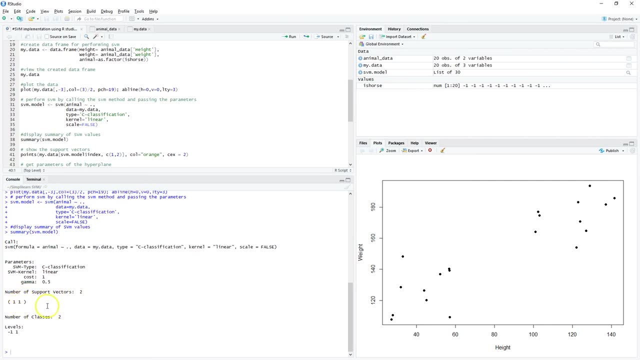 linear model and we've run it and great, now we have a model. let's look at the summary of the model and, as you can see, there's the formula that it ran and some of the information about the vectors in the classes, and there are two support. 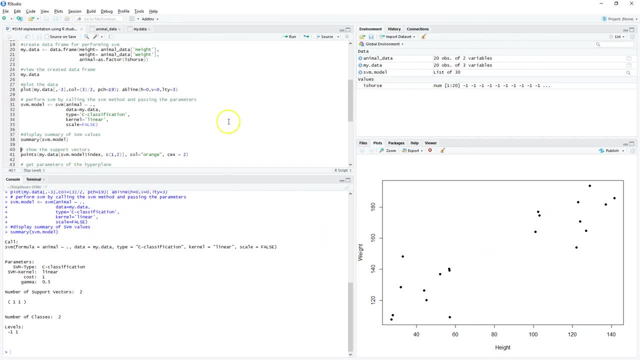 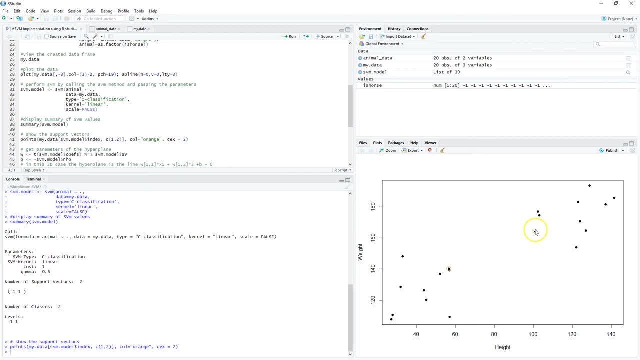 vectors. so now let's find those two support vectors. on our graph- and this might be a little hard to see- the orange outline around this point and this point indicate that those are the two vectors that will support this model, and thus we call them the support vectors. now let's get the parameters of the hyperplane. 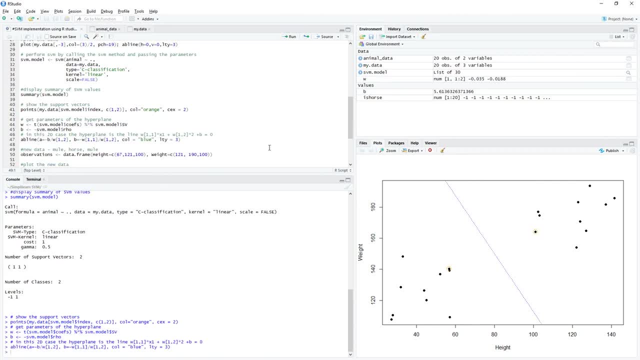 from the model. let's plot a line that will be our hyperplane. There's our hyperplane line and therefore, to the left and below are mules and to the right and above are horses. above that line, Let's take a few new observations and I've encoded these so that it would be illustrative. We'll take these. 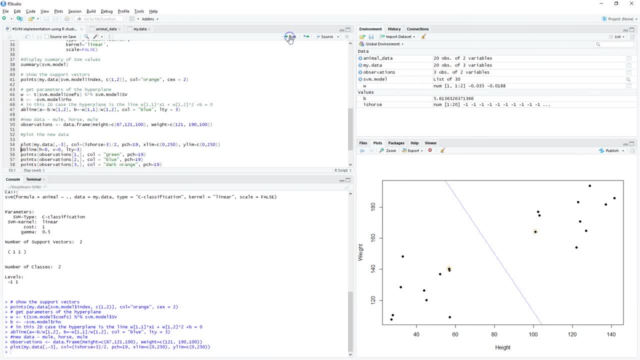 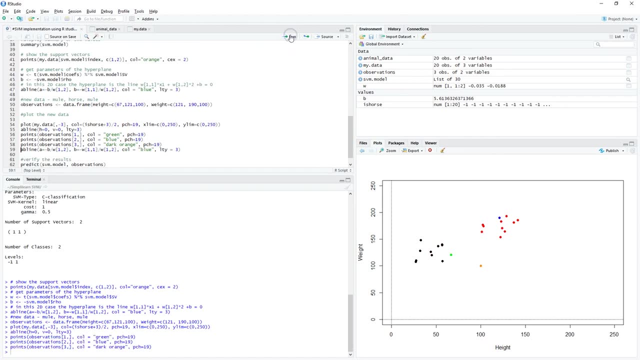 new observations and we'll plot them and I'm going to generate a new plot, red being the horses, black dots being the mules. I'll create an x and y axis. I'm going to plot three dots and you can see one of them, the green dot. the first, one kind of falls near the mules. the blue, one kind of falls near the. 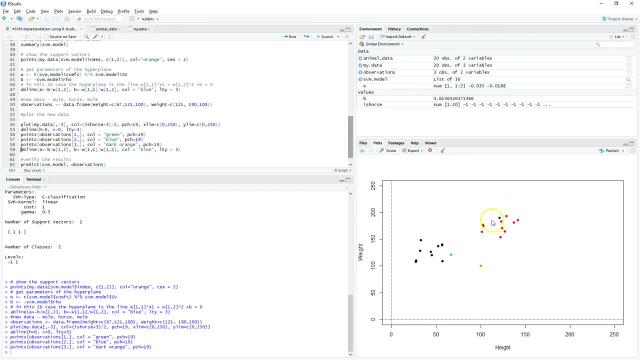 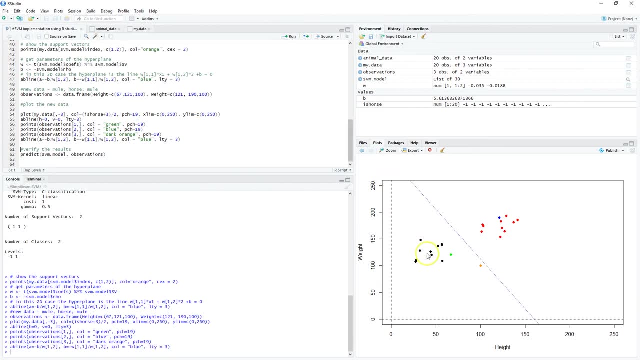 horses and visually we might conclude, hey, one's a mule, one's a horse. but what about the orange dot? well, for the orange dot, we really need our hyperplane, we really need something to clearly indicate which side it's on. and, of course, by looking at this data visualization you can tell. 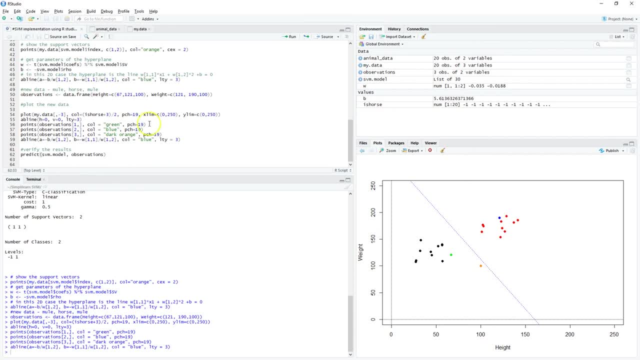 that the orange dot is the horse and the blue dot is the horse. So we're going to plot three dots is probably a mule and let's verify those results by sticking those observations into our model and predict some outcomes. and down below you can see that for the three data points one, two and three. 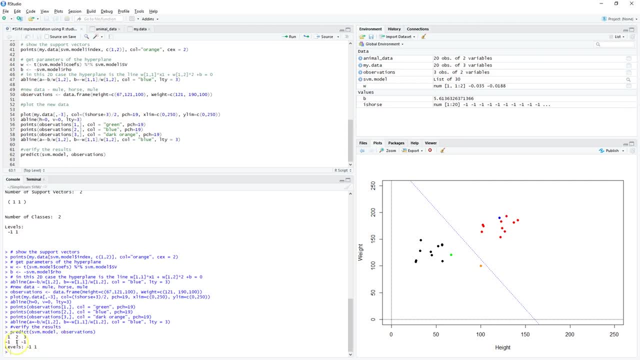 the first one. the green one was negative one, that's a mule. the second one was a positive one, that's blue. that's the blue point which was a horse, and the third one which we weren't sure about, but clearly the SVM model correctly predicted that that third point would be a 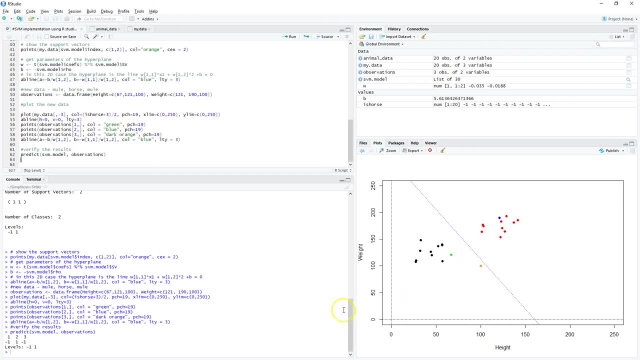 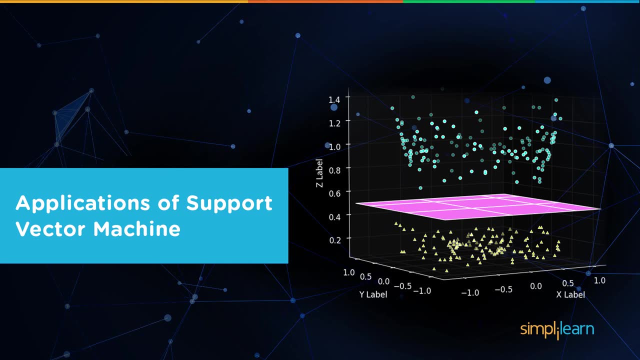 negative one would be a mule and we can see that the first one is a mule and the second one is a mule and we can visually see that by the hyperplane on the graph. So that's a quick example of SVM in general. support vector machines are binary classifiers. we don't use them for.